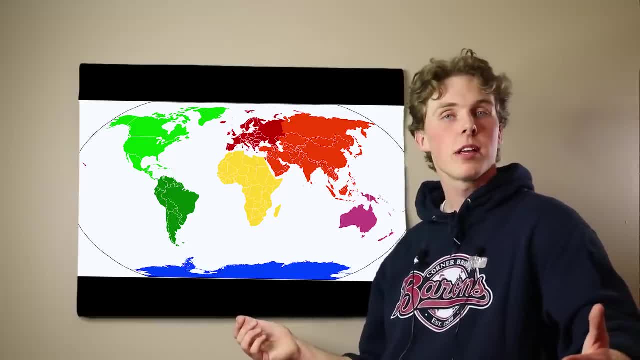 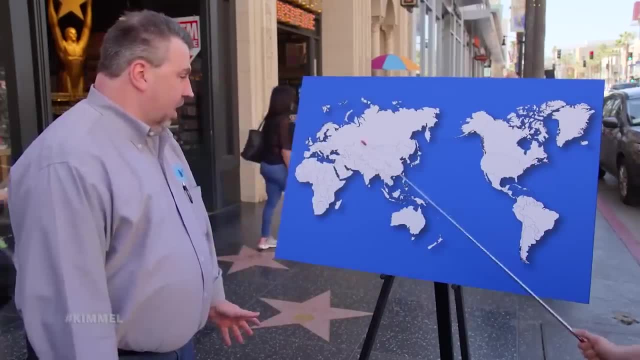 Like they can't even name one country. Have you seen those Jimmy Kimmel videos where he's like, hey, can you name a country? Somebody does? Africa, Russia, Nope, that's China. Europe. Where's Europe? Yeah? 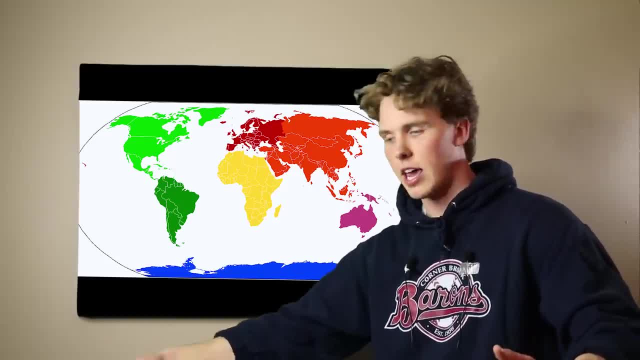 It's not like he goes into a young child's classroom and is like, hey, show me where Burma is, And then they can't do it. It's like, well, no shit, I don't know where Burma is, Jimmy. 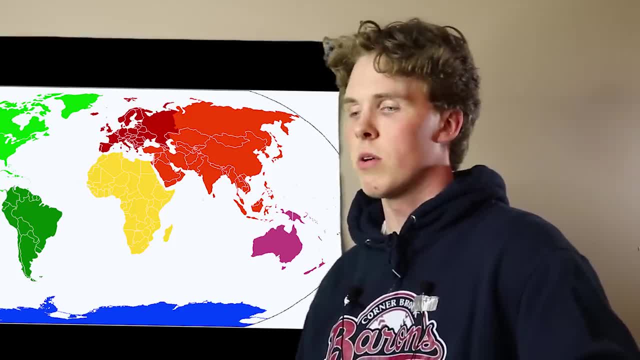 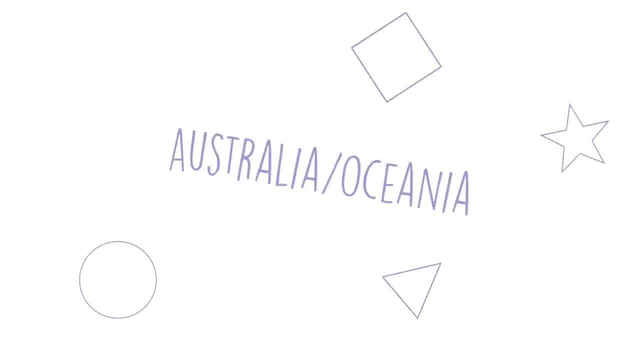 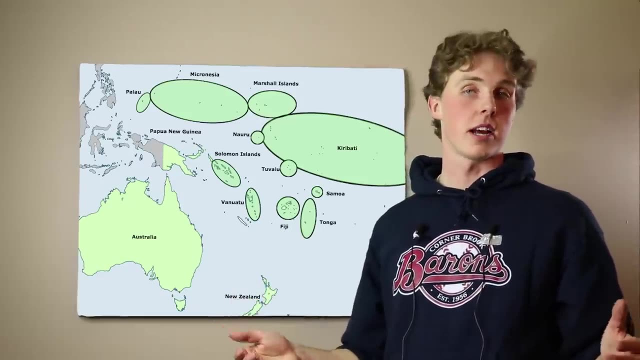 The only thing I know about Burma is that this morning I Burma-tongued on my hot chocolate. A very common misconception here is that Australia is the only country in the continent of Australia. And it's not. there are 14 countries there, all right. 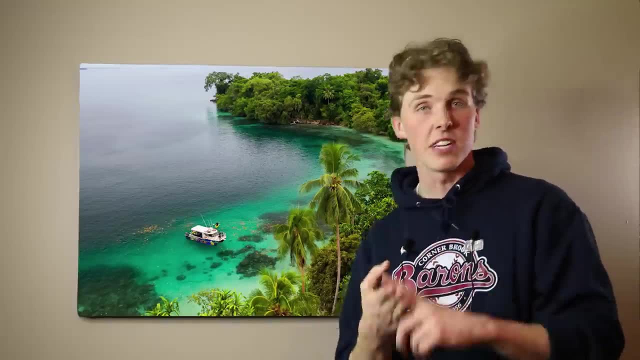 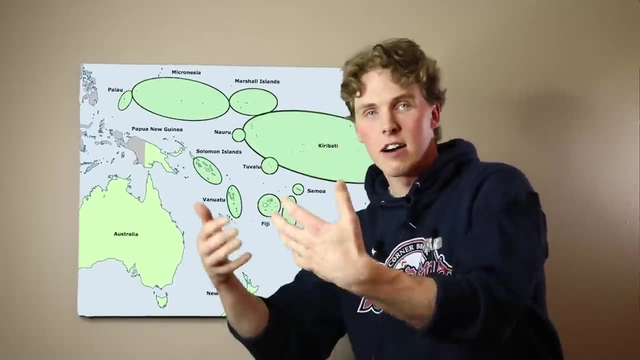 New Zealand's one of them. Papua New Guinea is one of them. you've probably heard of Fiji and Samoa. You've heard of all those. maybe Australia is a country in the continent of Australia. It's a little less confusing to call it Oceania. 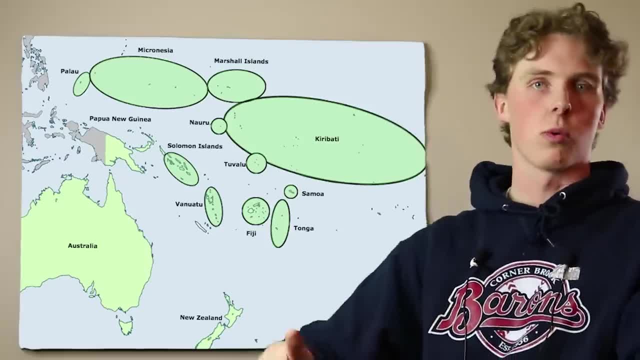 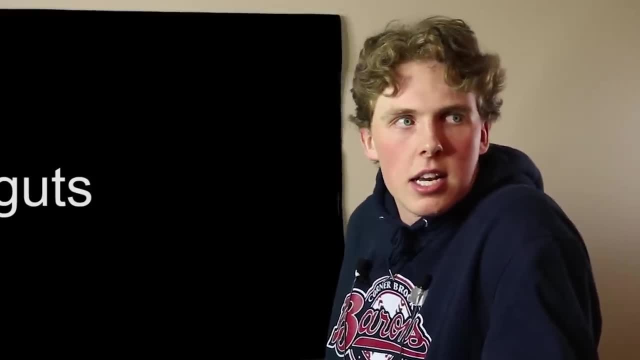 And it's a lot more fun to say Oceania, just like the word guts. You ever said that word, Guts, Say it right now. Any questions? No, Okay, If you look at the news at all, you probably know that Australia was recently ablaze. 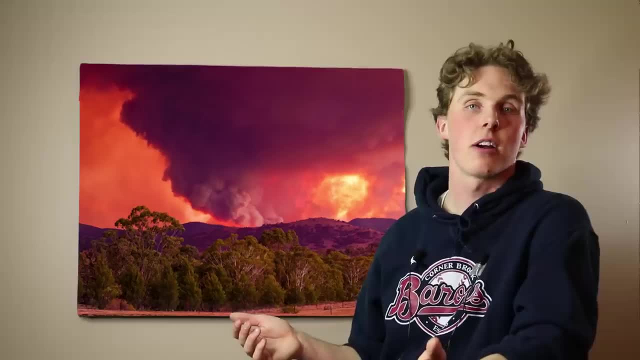 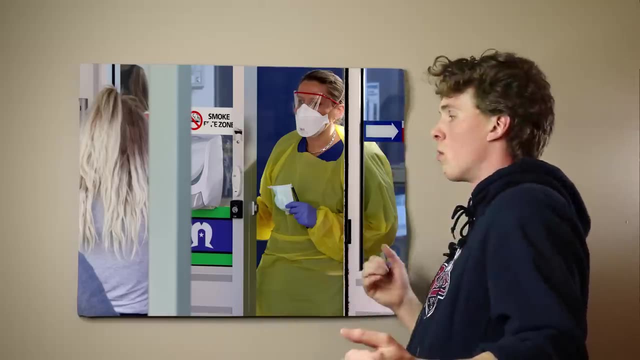 Almost the entire flipping country was on fire, And now it's not, I don't think, But now it's also ridden with disease, like the rest of the world. So Australia is doing real well in 2020.. Let's move now up the ladder. 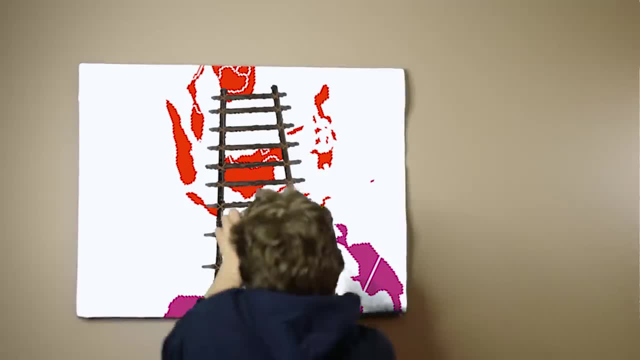 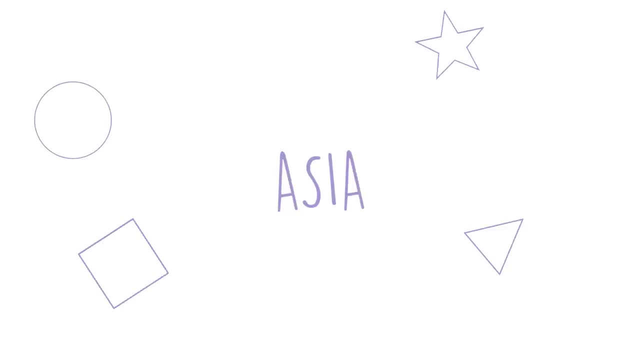 Let's climb it Ready like this. Hey guys just climbing the ladder, don't worry about me, That was fucking dumb. We're in Asia. Let's play some Asian music to set the mood for this entire segment of Asia. 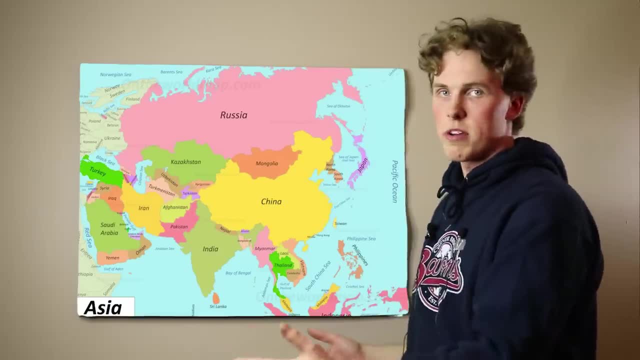 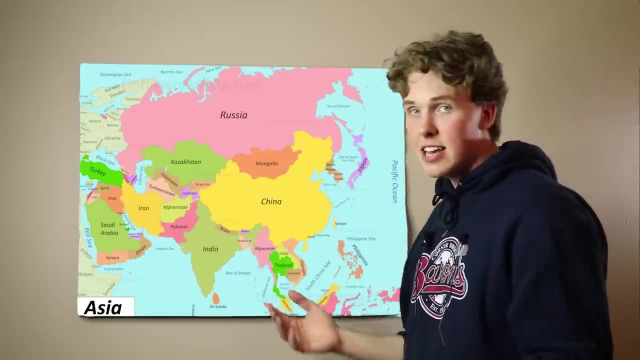 Welcome to Asia. One of the big players in Asia, I'm sure we all know China. okay, Another one: Japan, North Korea, South Korea, Russia, India. We all know about those big countries in Asia. okay, Those are the big ones, the big cahoots. 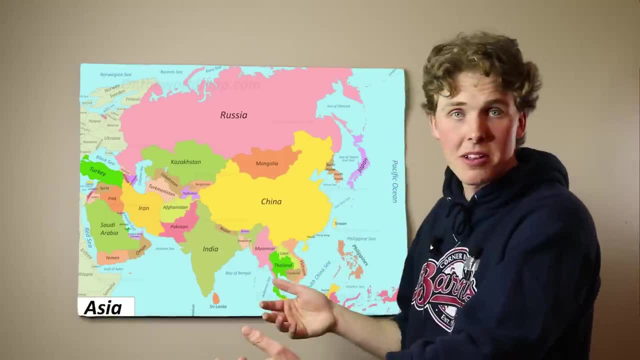 China has the biggest population in the world, with 1.6 billion, or something like that. Here it is now. That's what it is, I haven't been keeping up to speed. India also second with 1.1 billion. So a lot of people over there. One of the first things I ever learned was there are a lot of people in Asia. I woke up one morning when I was two or three and said: hey, dad, what's for breakfast? And he said: you know, son, there's a lot of Asians. 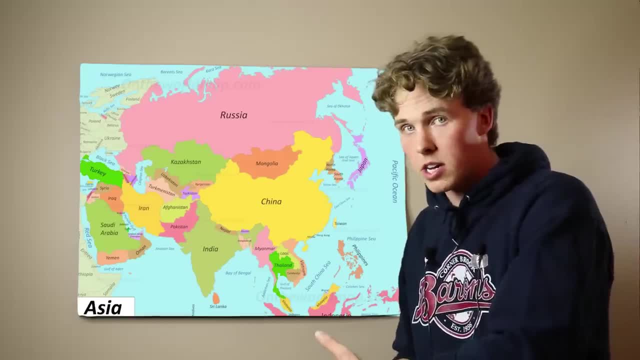 And I said, well, that's just about the first thing I've ever learned, dad. And then we had breakfast and it was great. And that was all a lie, obviously. But there's a lot of Asians. I like to split Asia into two. 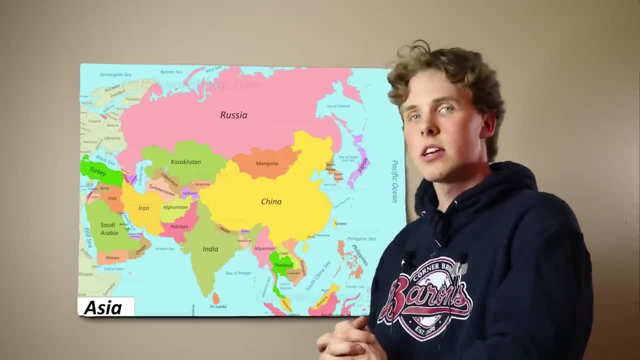 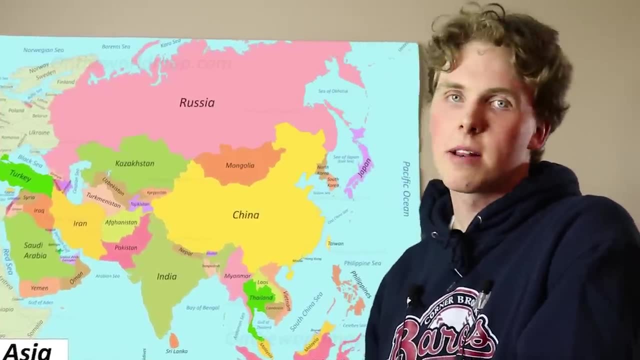 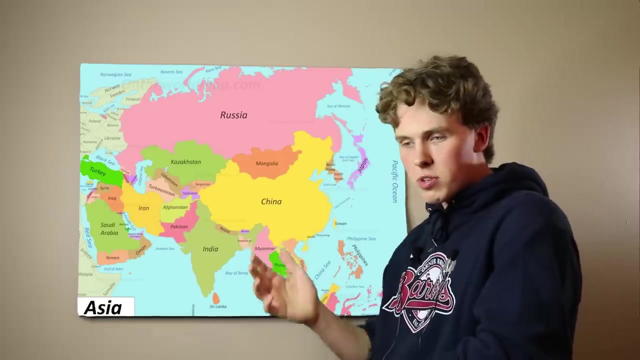 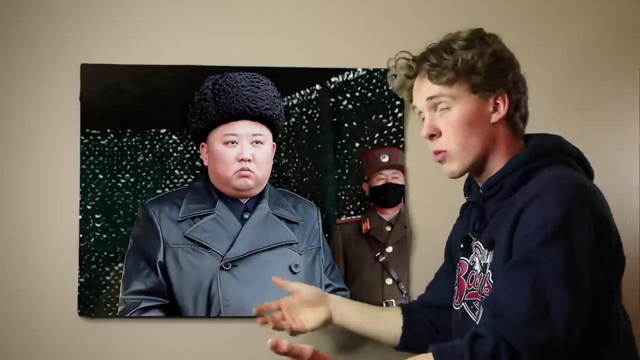 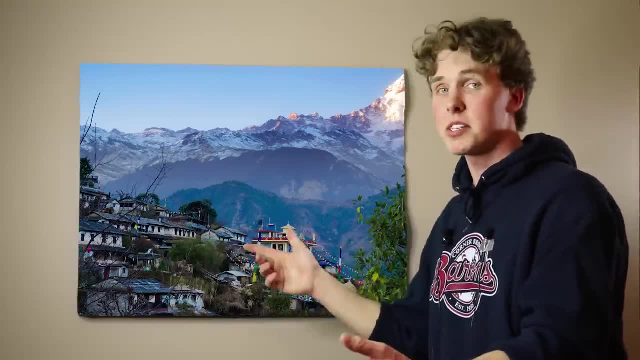 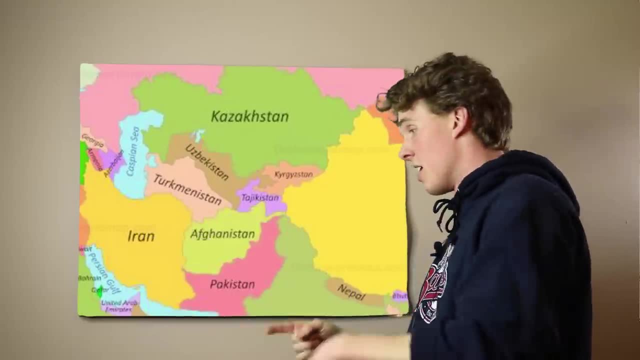 Indonesia, Singapore, Brunei, Bhutan, Nepal, where mount Everest is, and it sounds like nipples. What a country? What a country are the stands? all right, There's seven of them. We've got Kazakhstan, Kyrgyzstan, Turkmenistan. 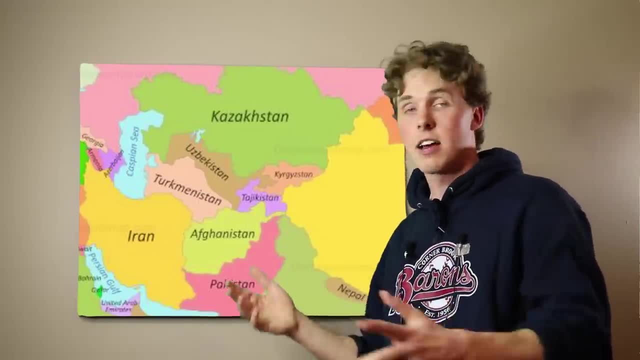 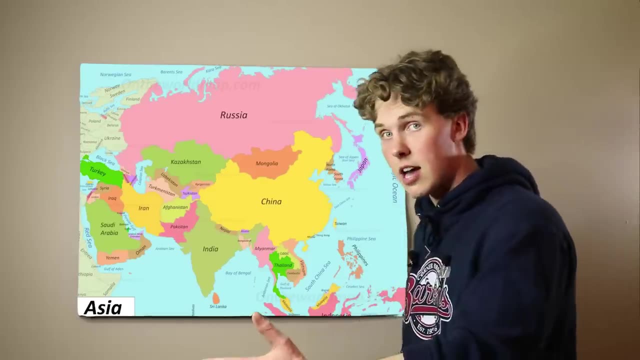 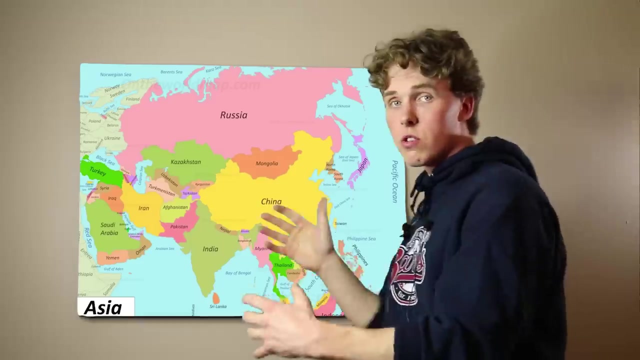 Uzbekistan, Tajikistan, Afghanistan and Pakistan. Let's not forget the K-pop stands. I'm not really big into all that lore because it seems to be a little toxic, a little too toxic for my pretty little feet- And boy, they're pretty- So I don't step foot in there, do I? Just to the west of the. 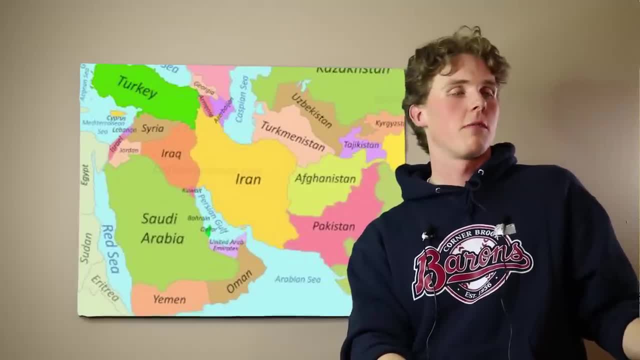 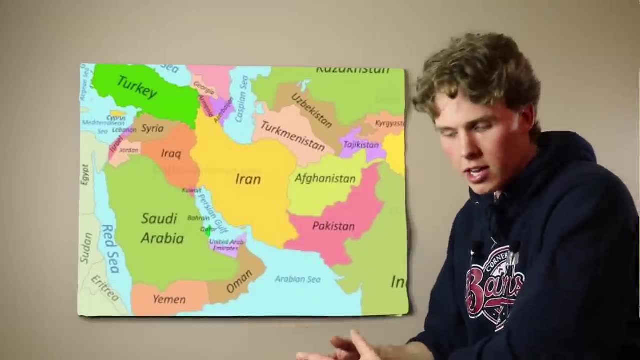 stands. we have the Middle East. The Middle East is, for lack of a better word term, war-torn. A lot of war goes on there in the Middle East, a lot of stuff going on, all right, You ever heard. 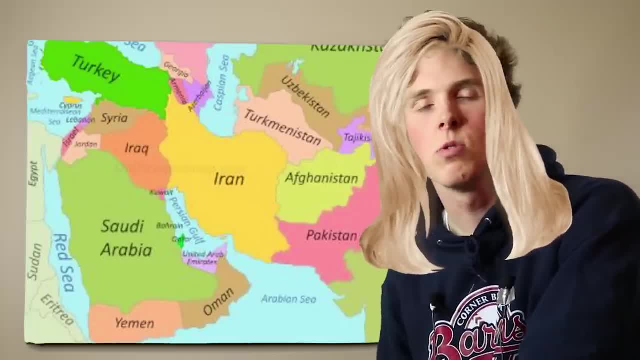 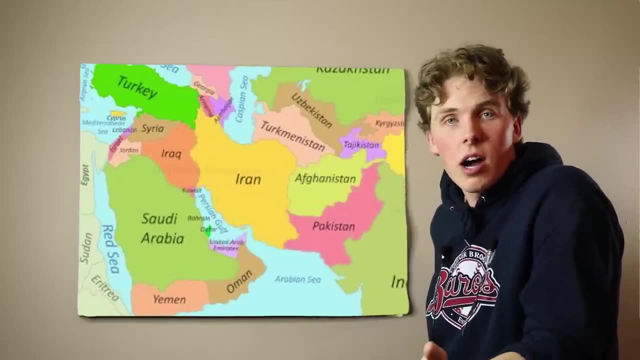 of jokes. It's like: oh well, I'll date you when you smooth out the Middle East. It's because there's a lot of conflict going on there. Maybe there's some good stuff going on in the Middle East. I don't know. Again, I don't know If you're from the Middle East and you're living a good one. 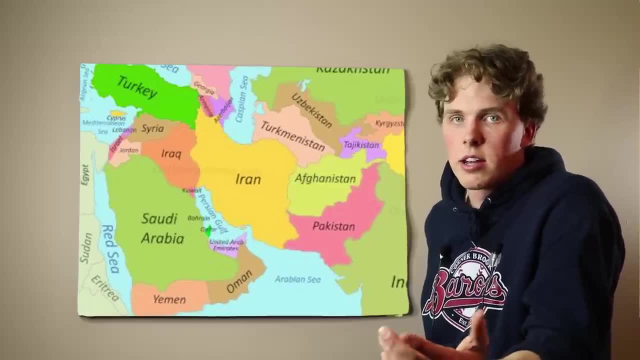 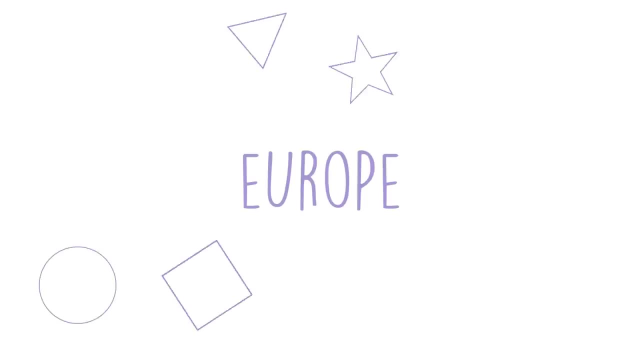 then you know, good on you, Good on you, mate. But if you're from the Middle East and you're living a bad one, not good on you. Have you ever heard of a place called Paris? You've seen the Eiffel Tower? You know, if you're? 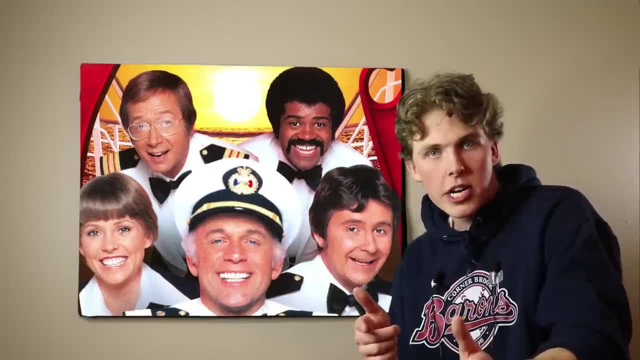 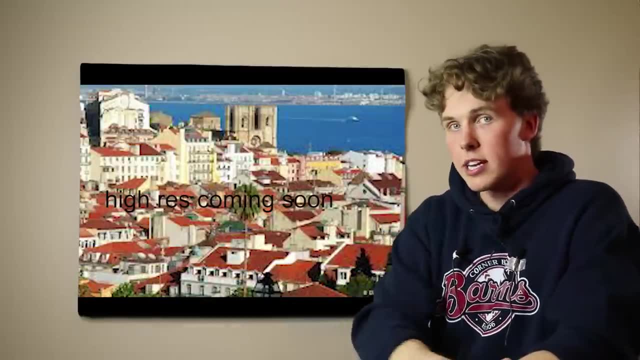 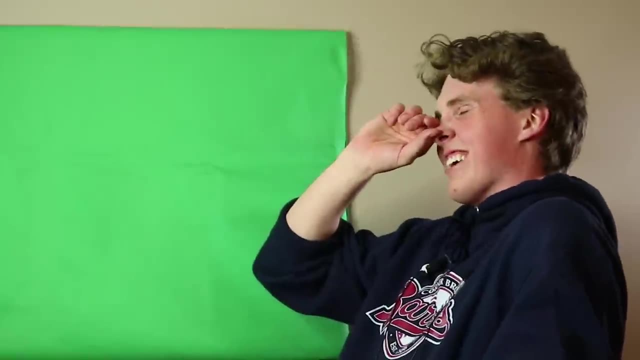 a love boat, you know, a little love boat, a little smoochy, smoochy. Valentine's Day coming up just 11 months away. Spain's there, and you've also got Portugal right next to that. Great spots of culture, lots of good art there, okay, Lots of good stuff. I don't know what the fuck. 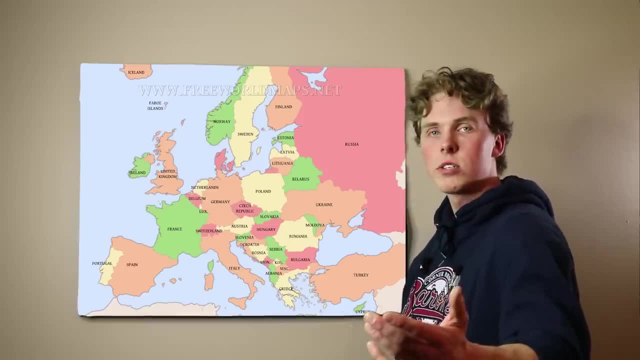 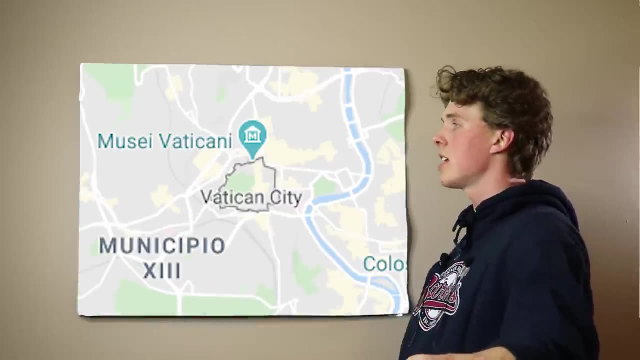 I'm talking about. No, but the countries are. some of them are way too small, aren't they? Countries like Monaco and Andorra and Liechtenstein and Luxembourg and San Marino and Vatican City, like the size of cities, And they're just countries Like fuck what? Maybe you know. 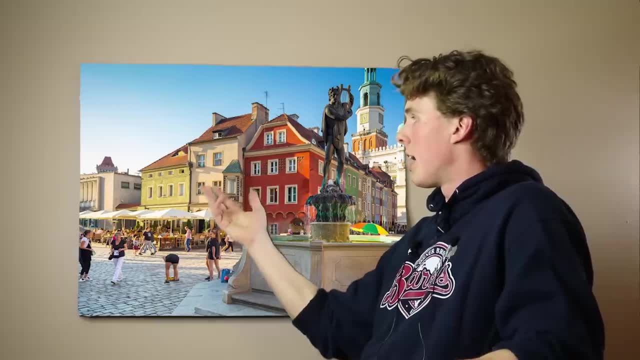 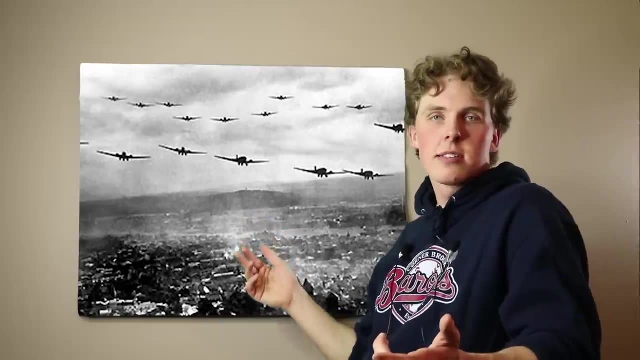 about Germany. Okay, that's a country, Poland, right next to it. You know a couple, you know 60,, 70 years ago they weren't the best of friends. Okay, it's over here, but now we'll. 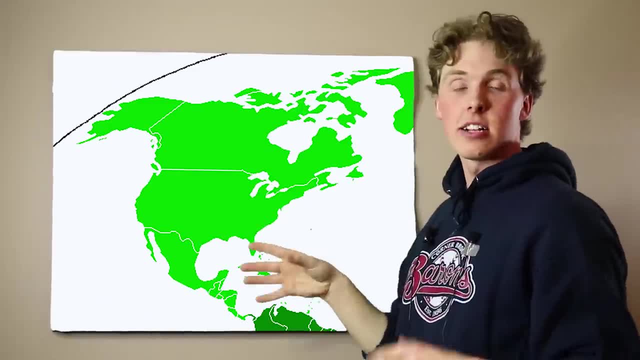 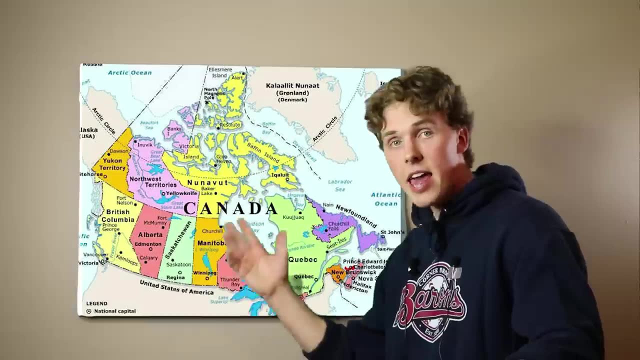 make it the full size, The screen ready. I'm in there, and so are so is 50% of my audience. So well, here you are, Welcome to North. well, welcome home. Canada, for example, has 13 provinces and 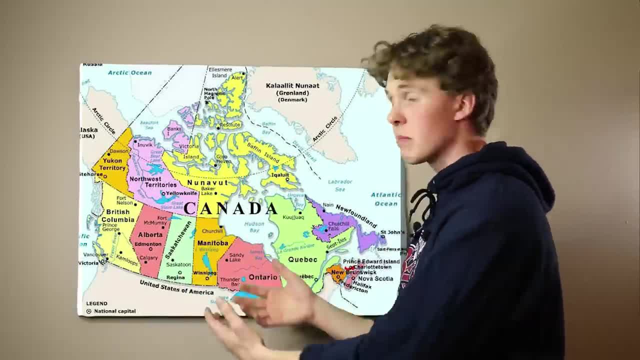 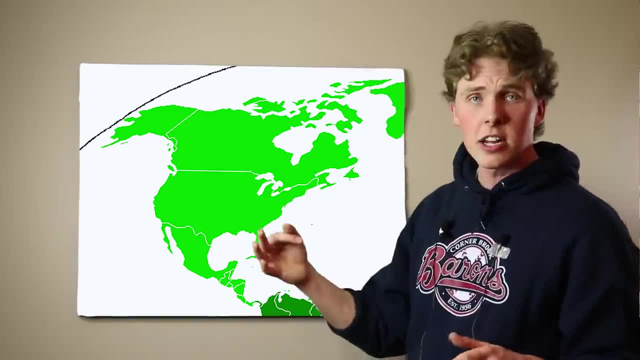 territories. okay, Newfoundland and the Labrador, where I am, is a province, as is Nova Scotia, Quebec, Ontario. A very common misconception with North America is that it only consists of three countries: Canada, the United States and Mexico. That's not true. It consists of. 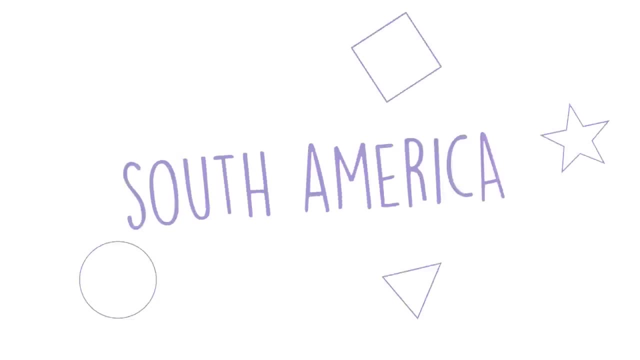 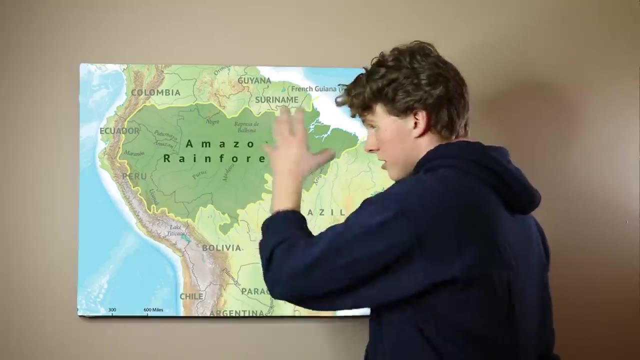 23.. Some time in your life you've probably heard of the Amazon rainforest. It's the biggest one in the world and that's in South America, And this is what this is where it is right there. See that It's mostly in Brazil, but I don't know what other countries it's also in. It might all. 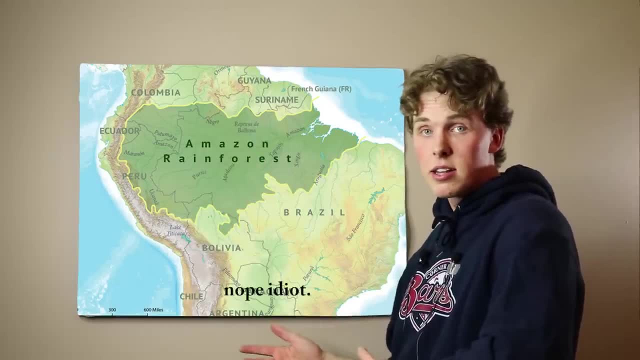 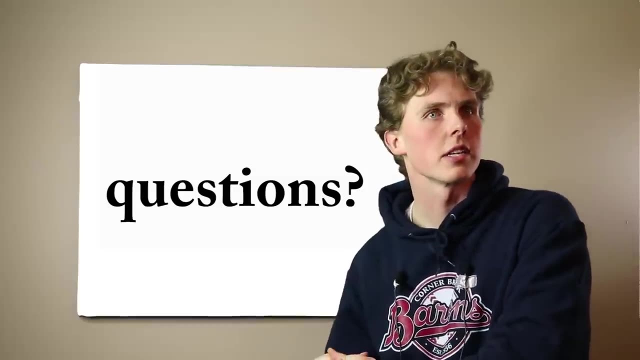 be in Brazil? I don't think it is, though Probably in parts of Bolivia, Paraguay, Uruguay- I don't know if it's in Uruguay or Argentina or not, but there it is. Do we have any questions yet? actually in the back? Yeah, yeah, Yes, I was a model before this. Yes, Teaching is something that 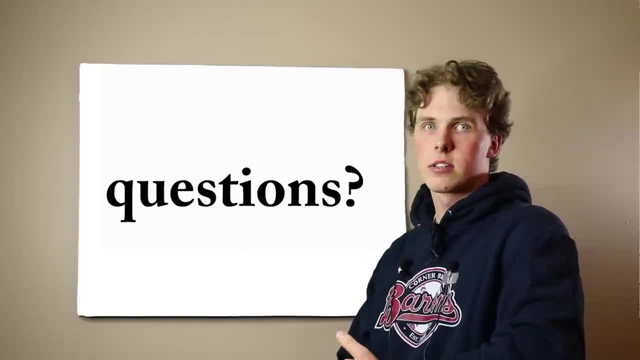 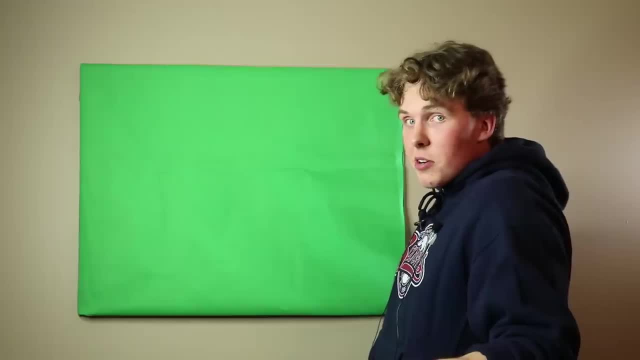 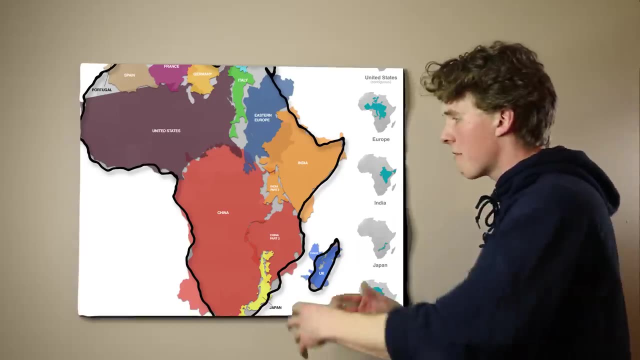 I kind of just, You know, happened into. I still have contracts for male sex work. Yeah, What the f**k am I saying My grandparents watch this. That's all you can do. hey, Got a silly grandson. It is a monstrosity. Look at how big Africa is compared to all the other countries. Look, 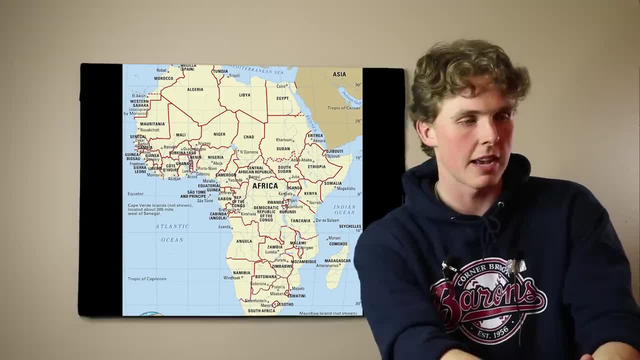 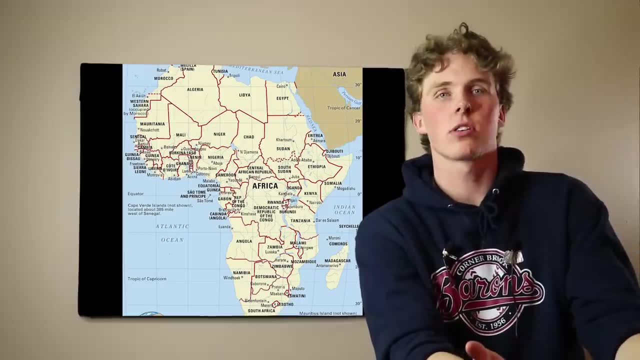 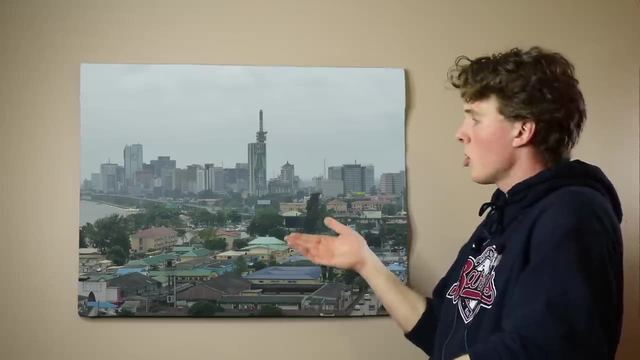 at how much you can fit inside of Africa. Look at this: A big misconception with Africa and I'll admit to this, I didn't really know this until, like I was in high school. Africa not all Dirt, grass and sand. Africa has cities like Cairo or Casablanca or Lagos or Johannesburg. 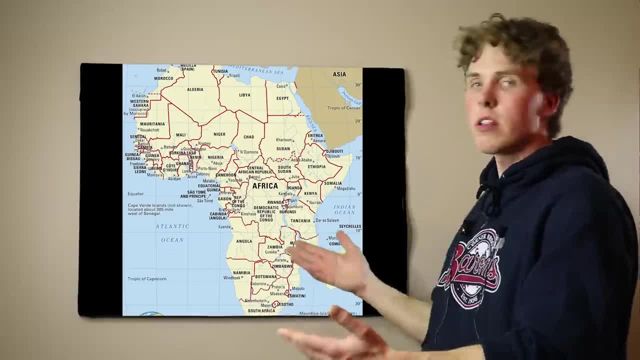 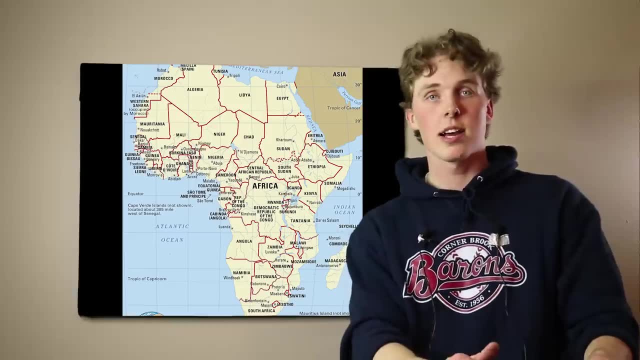 and Cape Town and Pretoria. down there in South Africa, People are living well there All right Now. certainly, certainly a lot of folks not living well there. Certainly a lot of poverty in Africa. Certainly a lot of dirt, grass and sand in Africa. Okay, You've heard of the Sahara. 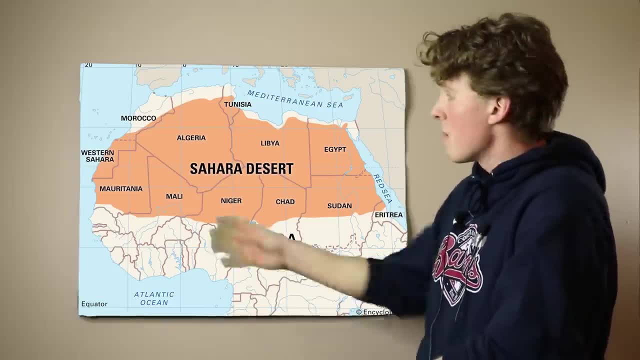 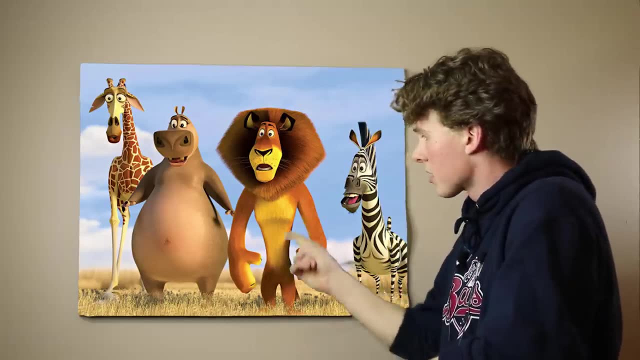 Desert That's over there in Western Africa. All right, Maybe it takes up more of it as well. Maybe it goes more in the middle too. I don't know where it is. You've heard of the movie Madagascar. Well, there's an island called Madagascar. You probably knew that. If someone's 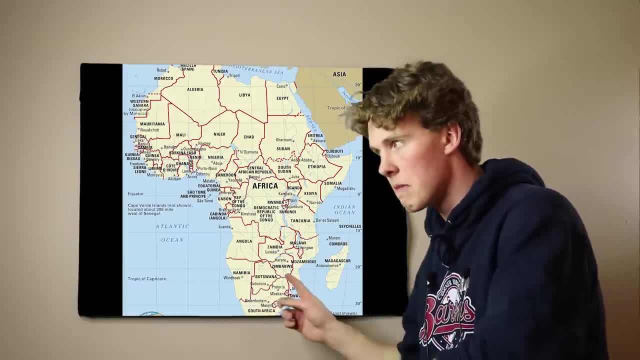 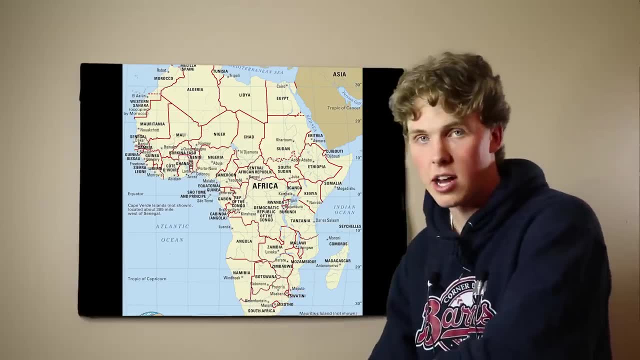 like, let's try to name all the countries in Africa. you're like: huh, I've got one: Madagascar, We're off to a blazing start now. 53 left. Good luck, South Africa, that's one, and you're stuck. Okay, Let's rhyme a few off for old time's sake. Okay, Namibia, Botswana. 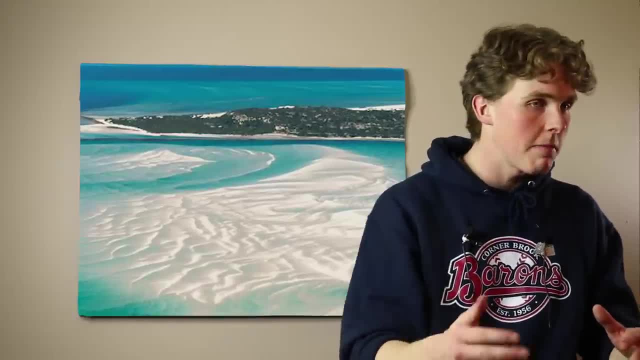 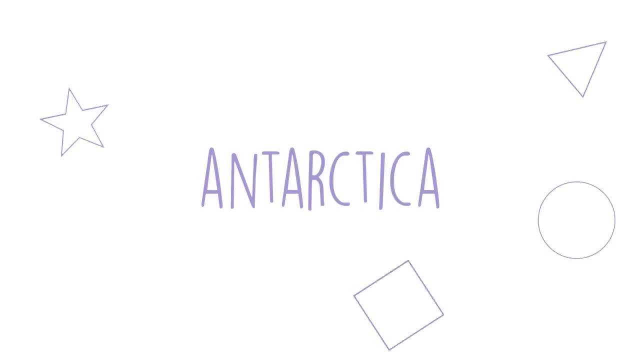 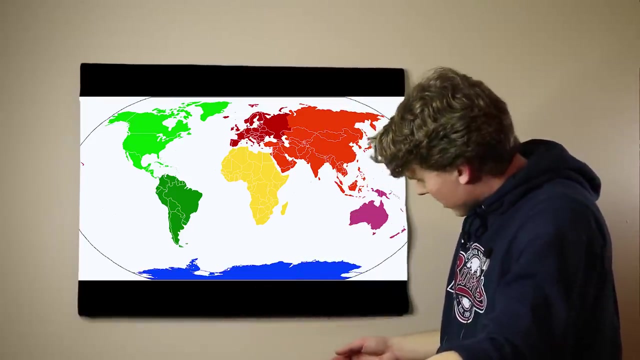 Gambia, Ghana, Gabon, Zambia, Zimbabwe, Mozambique: You a fan of Apex Legends? Mozambique? yeah, Lay in some cover for my brothers. Yeah, that's it, That's all Well. Antarctica: How could I have forgotten about Antarctica? 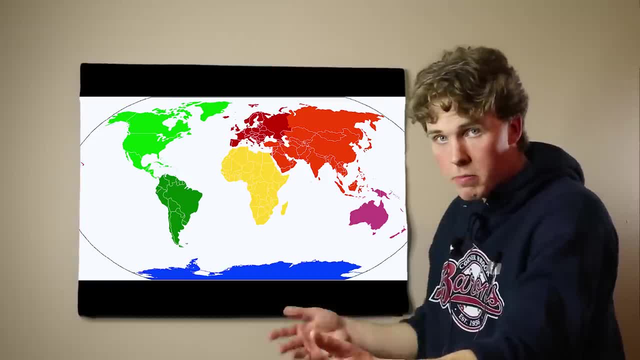 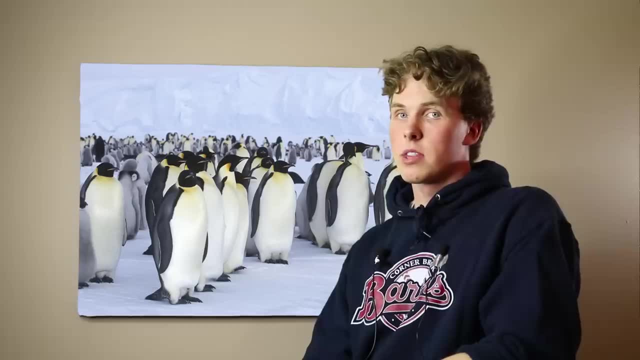 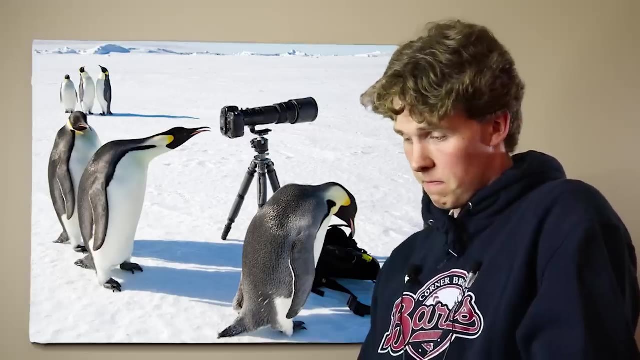 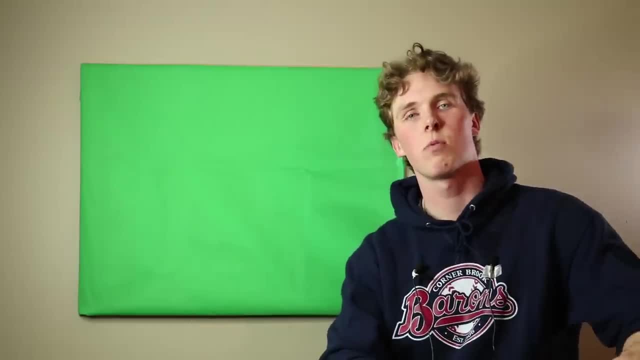 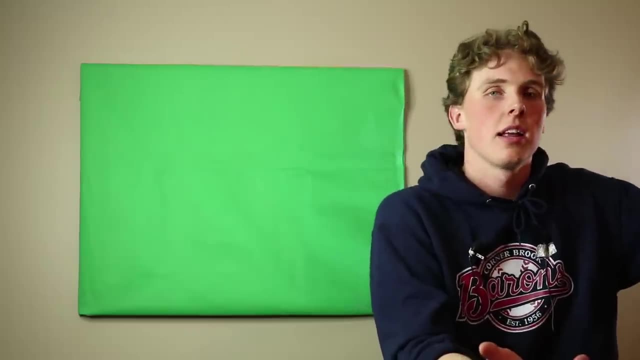 I am not a idiot. I have nothing else to tell you. Okay, thank you so much for watching. If this is your first video of mine that you've watched, or if you've watched a few and haven't that red subscribe button down there yet, go ahead and do that. That'll be really cool. 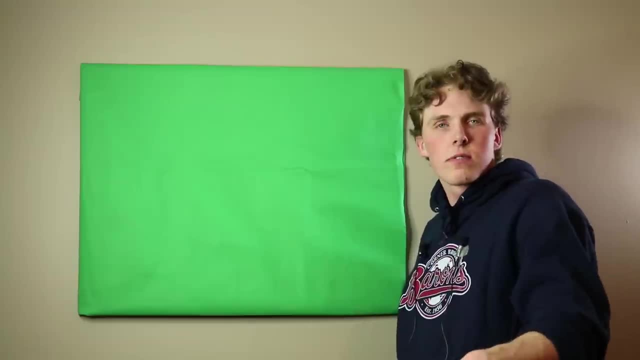 I'd really appreciate it or at least consider doing it. This was all for goofs, for goofs and gags. If you didn't know these things, that's fine. Hopefully you learned something. If you did know them, that's also great, Hopefully. 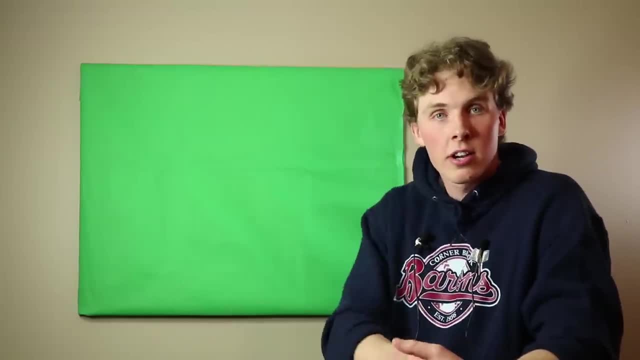 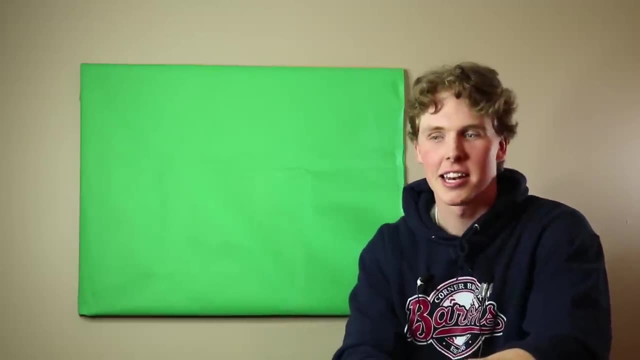 you maybe learned something too. Maybe there's something a little givlet, a little nugget you learned in there. Nugget's the fun word to say, But yeah, that's it. Don't forget to subscribe. Thank you very much for watching again.